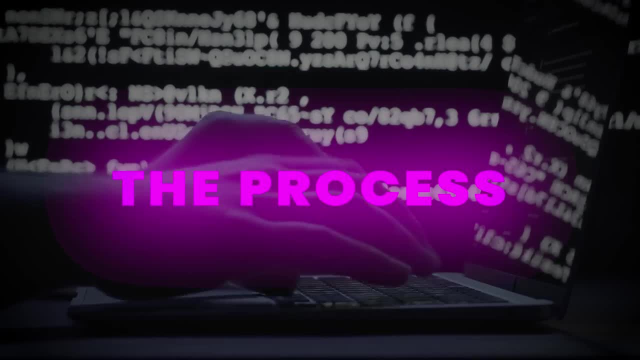 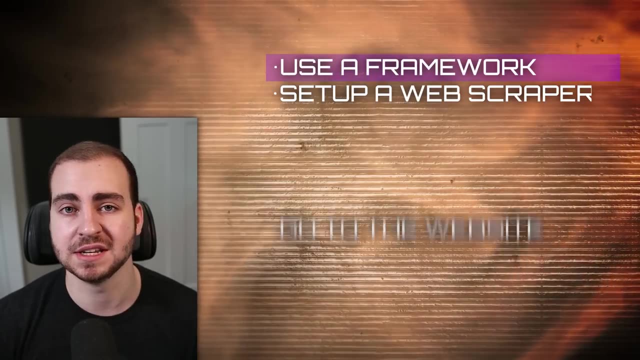 start tracking their prices and alerting me or my clients of any changes in those prices, such that we could react and modify our prices so that we could take advantage of an opportunity. Now, before I did all of this, I did ask my community if they had any advice on how to go about building a 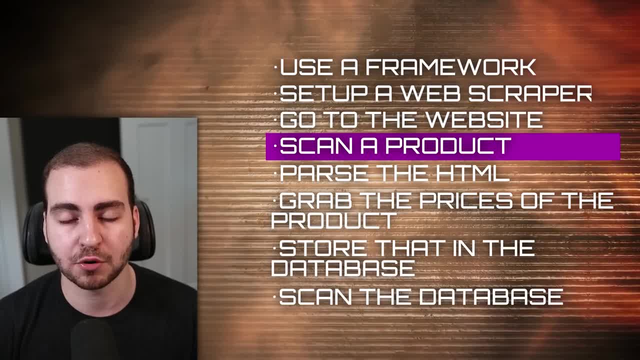 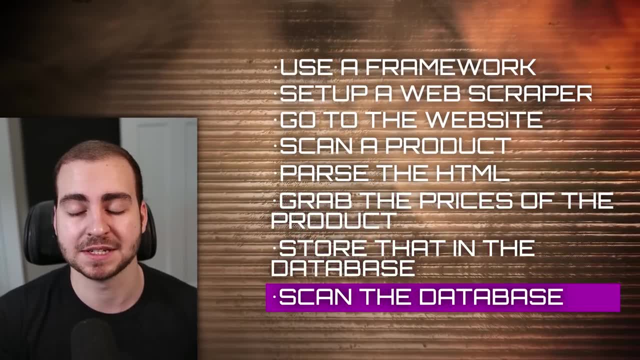 project like this. What they suggested is to use a popular framework like Playwright or Selenium, set up a web scraper, go to the website, scan for a specific product, go parse the different HTML, store that in a database and then scan the database and see if there's been any changes. 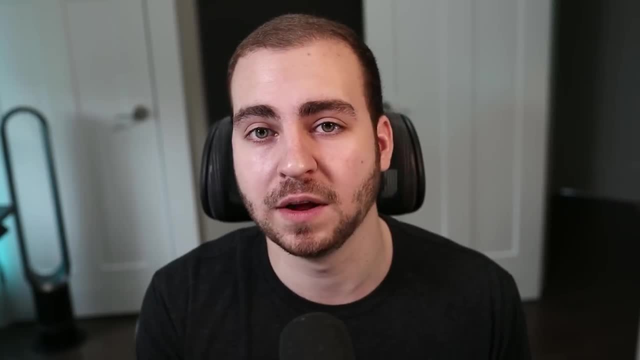 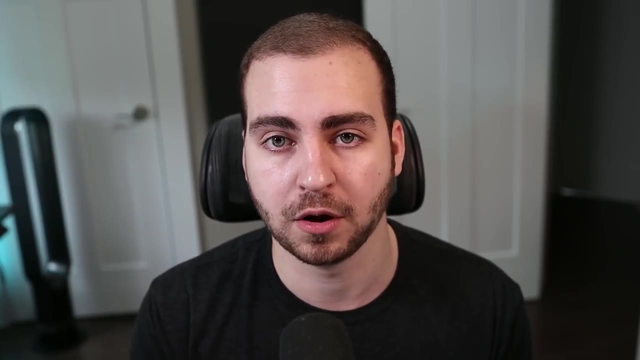 since the last time we updated that product. They then said I could run the scanner automatically at a set increment, So every day, every hour, every minute, whatever increment I choose, and that would be how we can work on this project. Now, unfortunately, every time I attempted to do, 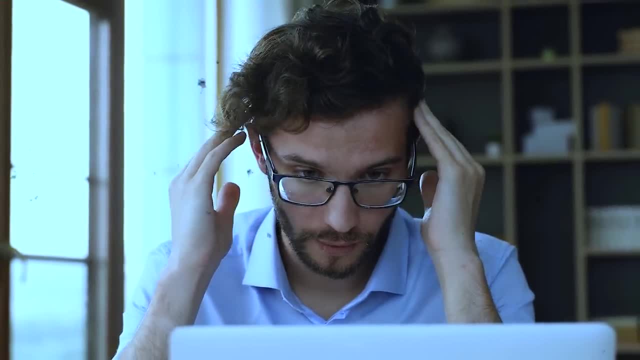 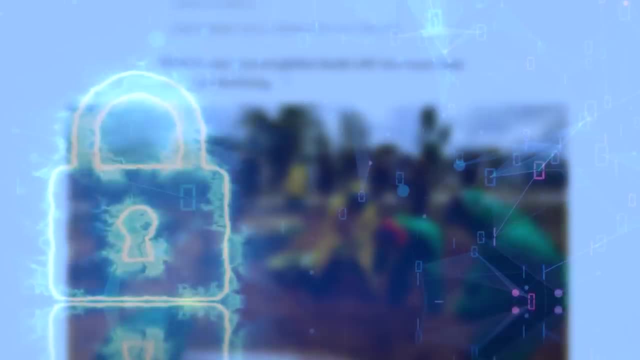 this. my IP address got blocked, I got stuck behind captures and I just got completely denied and shut out of the website after just a few attempts at scraping it. Now it turns out the websites are pretty smart. They can detect bots and they really don't want you scraping their 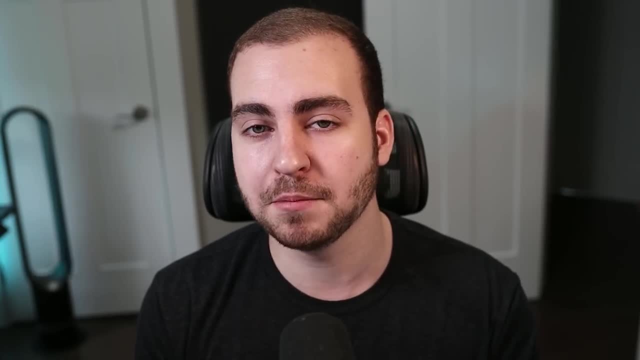 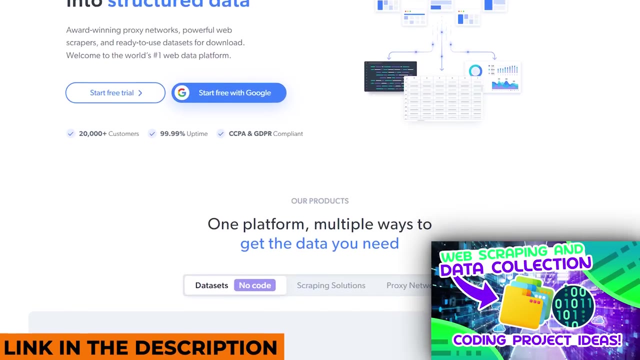 website and doing exactly what I was attempting to do. Now that's what I remembered: that about a year ago I'd worked with a company called bright data. Now bright data essentially unblocks your browser for you. It'll automatically solve captures and all that kind of stuff. 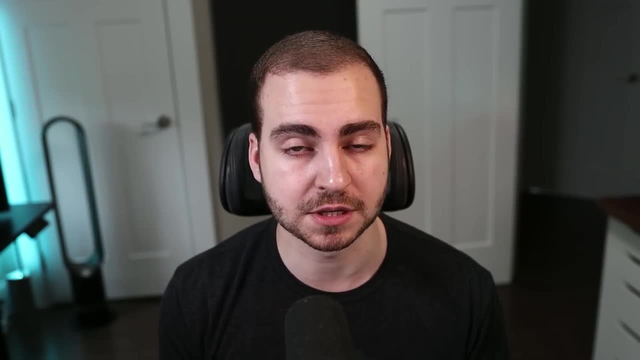 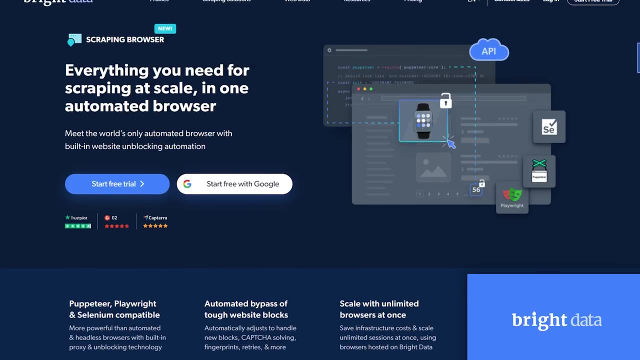 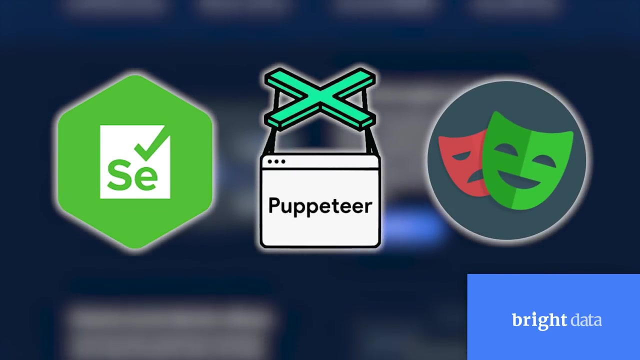 So I reached out to them. we connected and they agreed to sponsor this video so that I could continue building this project. Now what bright data gave me access to is something called their scraping browser, which is a head full browser that works with Puppeteer, Selenium and playwright and automatically unblocks websites for you. It will connect to a. 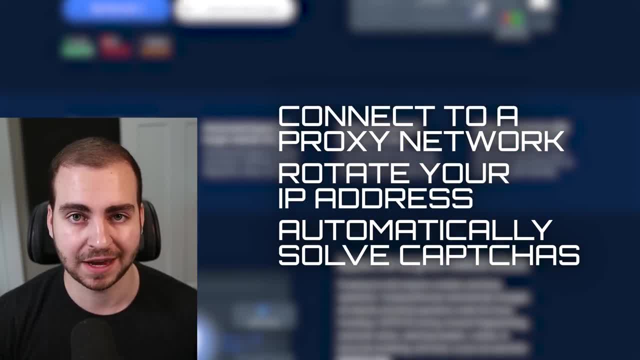 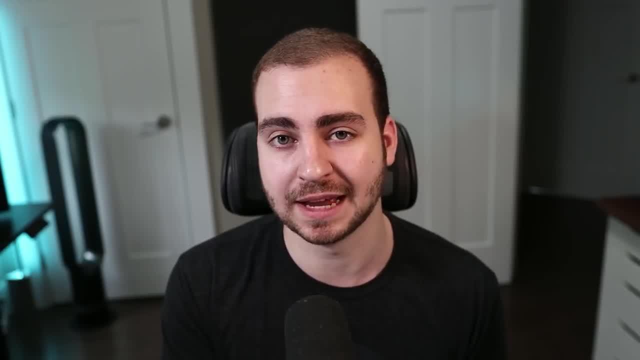 proxy network, rotate your IP address and automatically solve captures, essentially allowing you ungated access into a website and to perform web scraping. Now, most importantly, it also allows you to do scaling, meaning I could run hundreds of instances of my scraper at the exact. 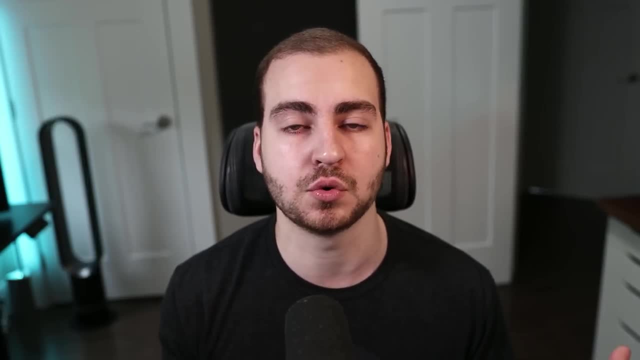 same time, And I wasn't limited to a single instance or whatever my local machine could handle. So that's what I ended up using for this project. I'm going to show that to you in a second, but if you do want to check out, 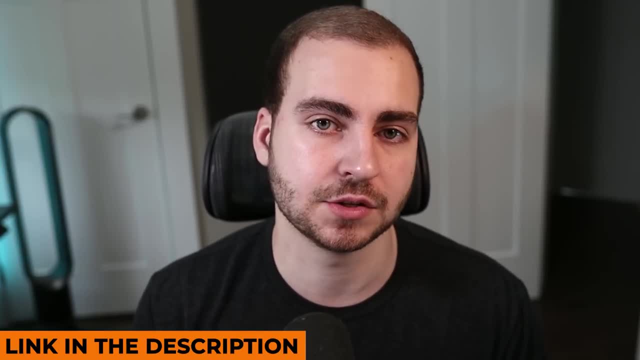 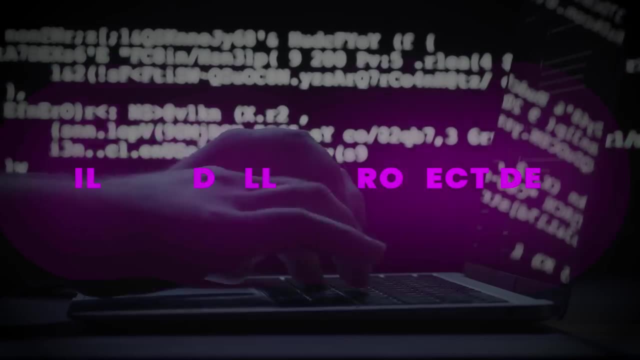 right data. they are the sponsor of this video. You can check them out from the link in the description and you'll get access to some free credits that you can try this out for yourself and see the power of a browser like this. All right, So now let me show you the project that 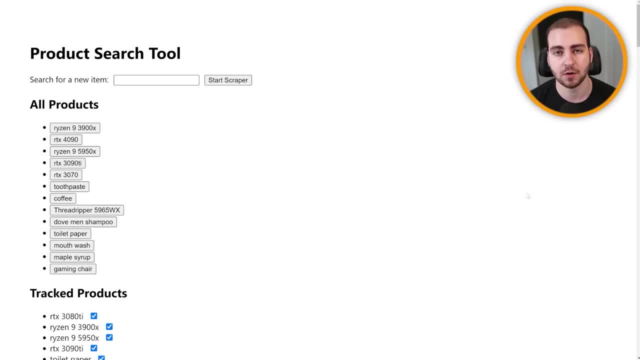 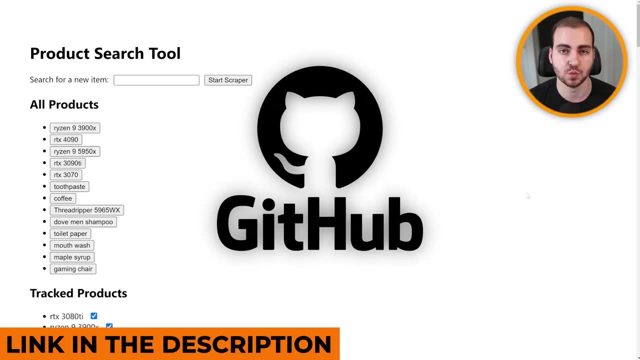 I actually ended up building That's fully functioning and working right now. If you want, you can extend this project. I'm leaving it completely open source, So click the GitHub link in the description and feel free to do whatever you want with this code. You can make. 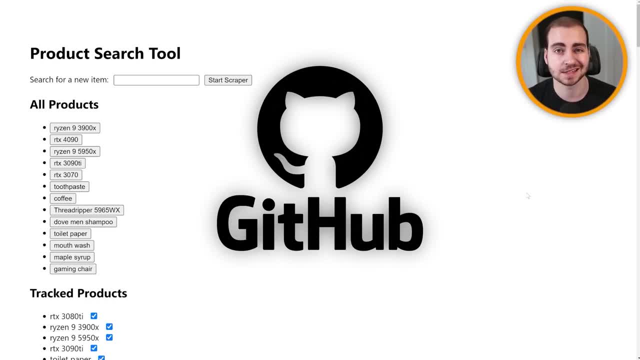 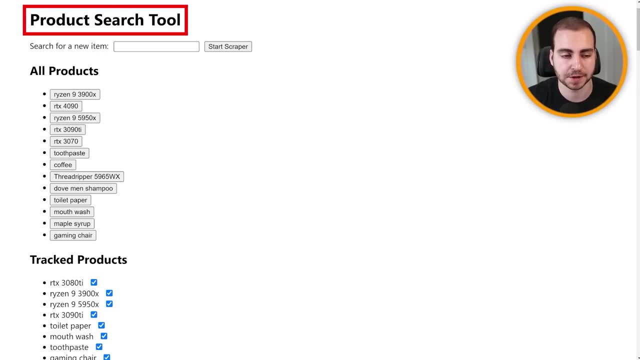 something really cool. This is kind of a solid base and you could extend this and make a legitimate business. Anyways, you can see that what I have here is a product search tool. Really, It's kind of analyzing e-commerce prices And right now it goes to Amazon and it will automatically scrape Amazon every. 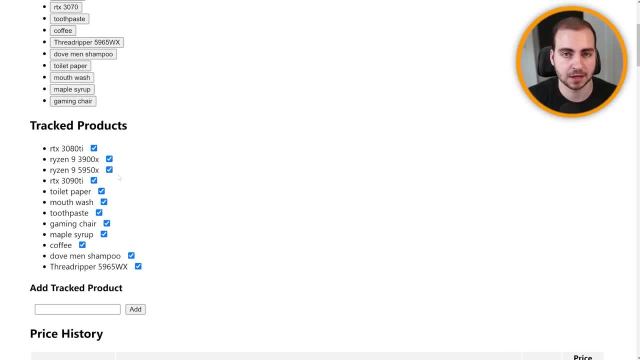 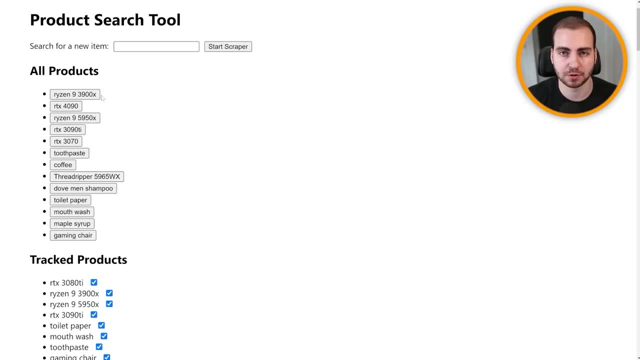 single day for all of the different products that I have that are set up here. So I can either enable or disable tracking of this product. I can add a new product that I want to track and then I can view the individual prices for these products. So let's click into rise and nine, 59, 50 X, That's. 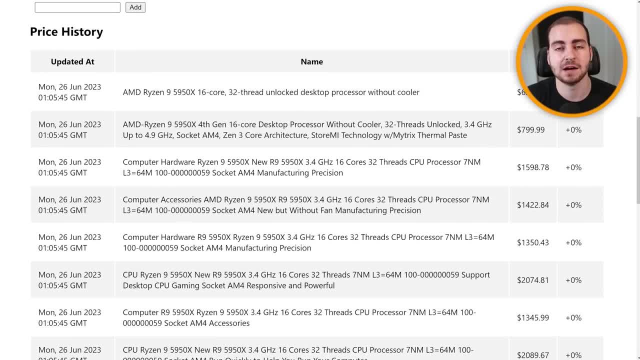 going to generate a table for us down here of all of the information we have on this product currently from amazonca. Now you could scrape multiple sources at once, for right now I've just set it up to do Amazon, but you'll see the way I wrote my code. You can automatically add other web. 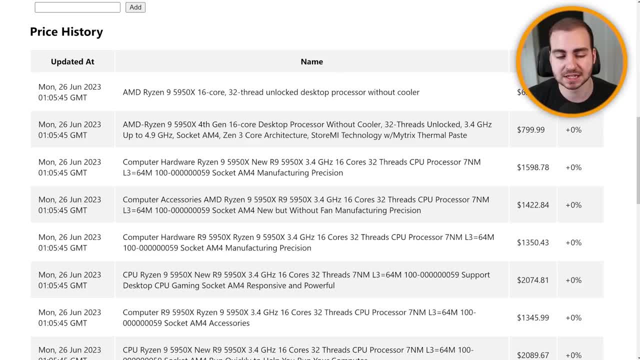 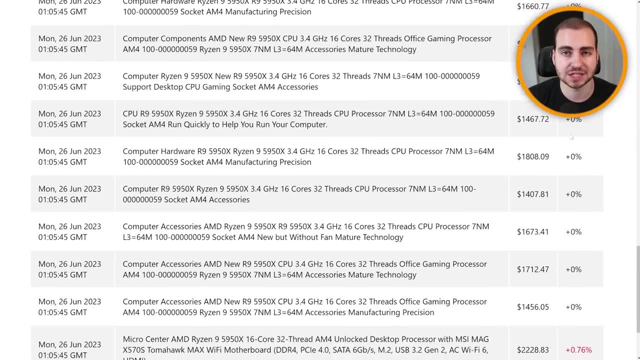 scrapers and set up different sites. Now it shows me all of the relevant listings that contain the rise in nine. 59, 50 X processor from Amazon gives me the current price and any price change since the last time the scraper ran. So you can see down. here we have kind of a combo of a CPU and a. 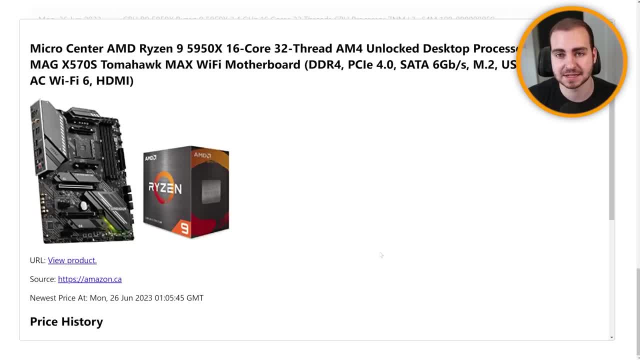 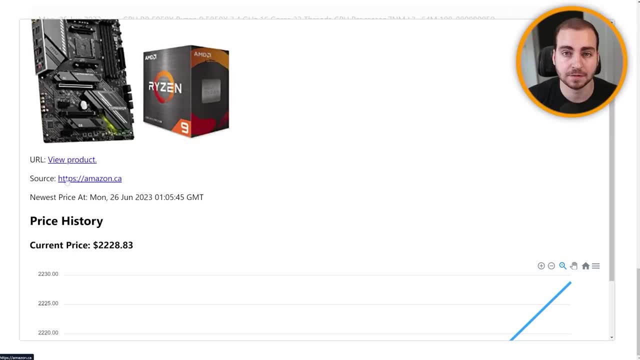 motherboard, and this has gone up 0.7, 6% since the last time I ran This. So you can see, here we have this micro center AMD. whatever gives you all the information. You can view the product URL, view the source- newest price, time, current price And then it. 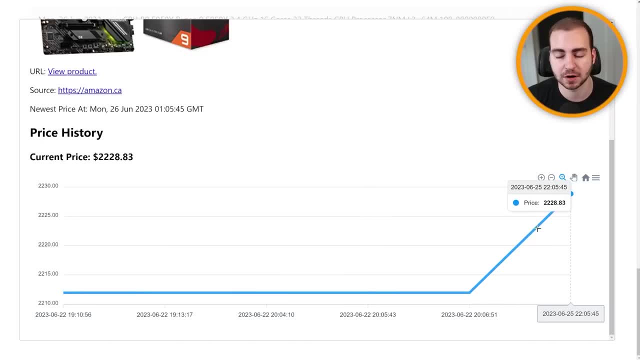 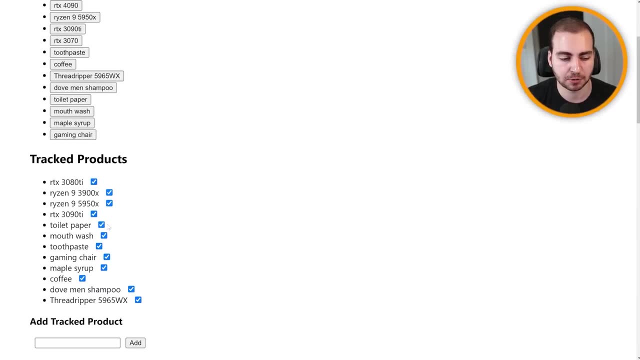 gives you a graph actually telling you the whole history of this product from when this web scraper has been running again. the way this works is: every single day, it automatically scrapes all of your tracked products and then gives you any updates on them. Now, you're not always going to. 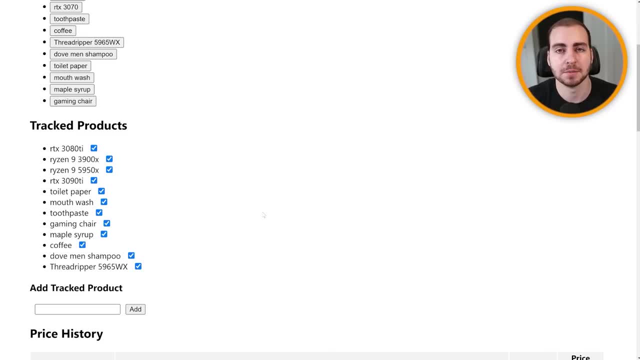 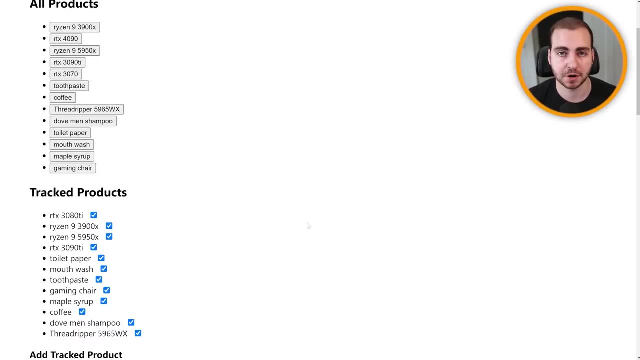 have a price change and it depends on how frequently you run the scraper, But in my case I've seen a few different changes. I was actually pretty surprised to find out that even large sites like Amazon are constantly updating their prices, And you can see. 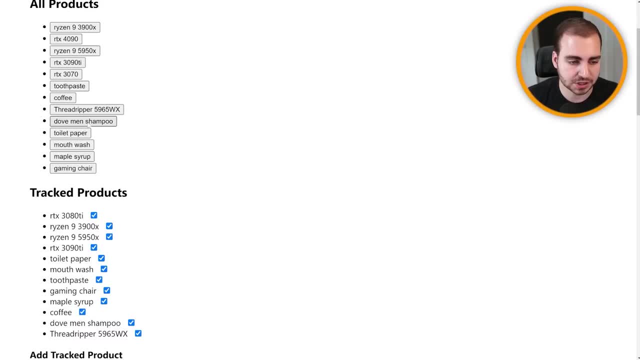 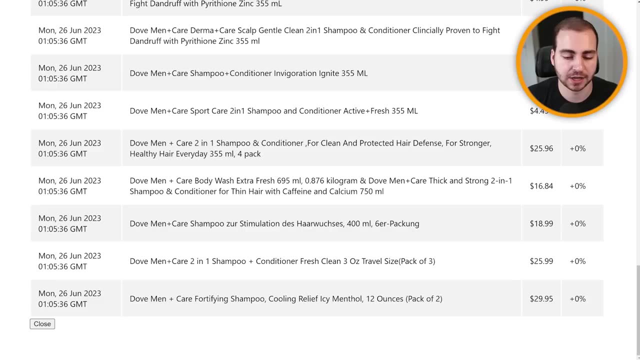 quite a few different price changes here, So we'll go into one more to see if there's any changes in something like dove men shampoo. Don't think we're going to see any here, just because this is a pretty basic kind of product And I only actually ran the scraper one time, So that makes sense. We wouldn't. 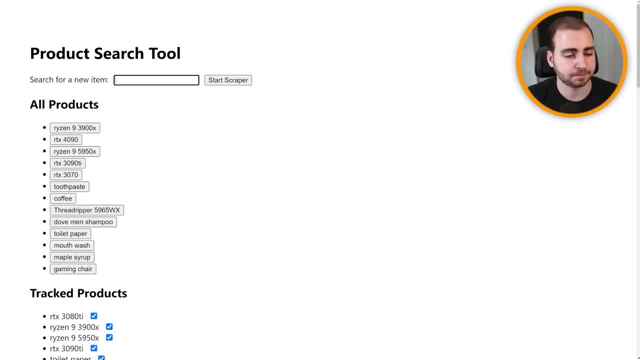 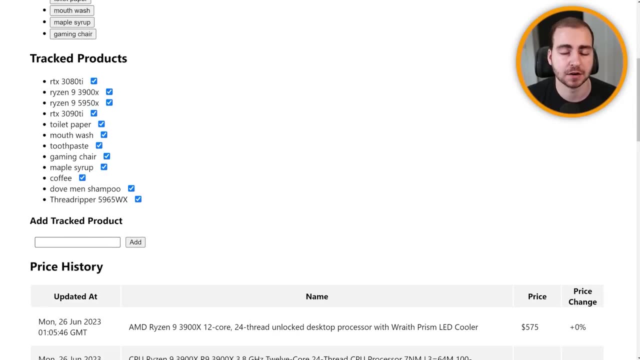 see a price change there And if I want I can even track another product So I can go up here and just search for one one time, or I can add it to my tracked product list to be automatically updated and ran every single day. So that's a pretty basic kind of product that I only actually ran. 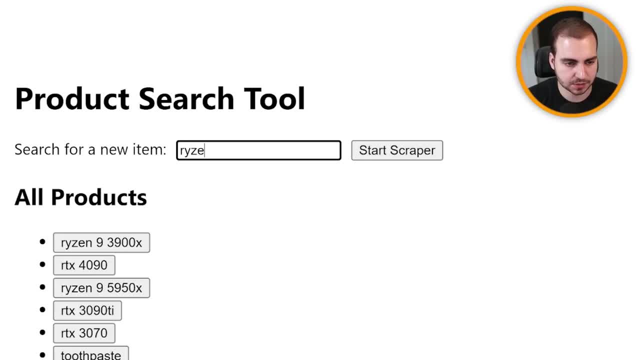 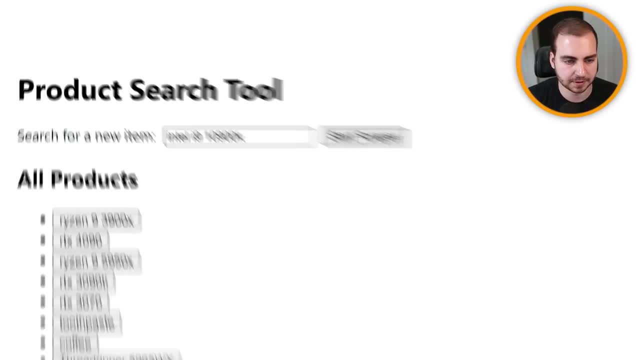 every single day. So let's just track a random product here. Uh, let's do something like Intel I nine, uh 10, 900 K- I don't know if that's recent or not, but let's scrape this, Okay. 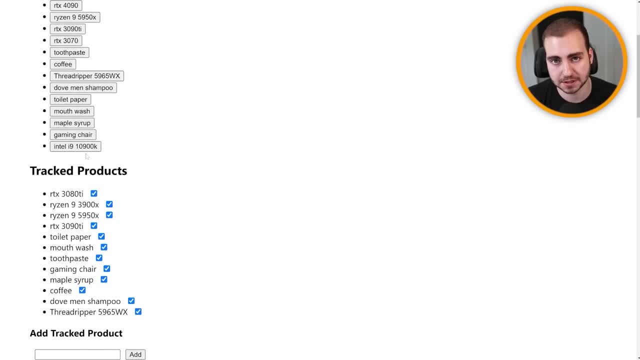 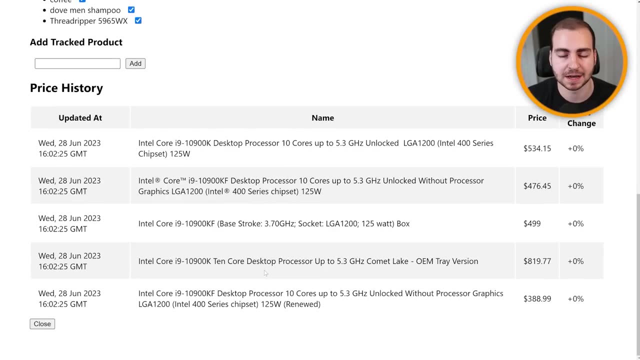 We'll give that a second to update and then I'll show you the table that it generates. All right, So this is finished. So I'll click on this Now. gives me the table and shows me all of the different listings from Amazon that were relevant, that contained Intel I nine. 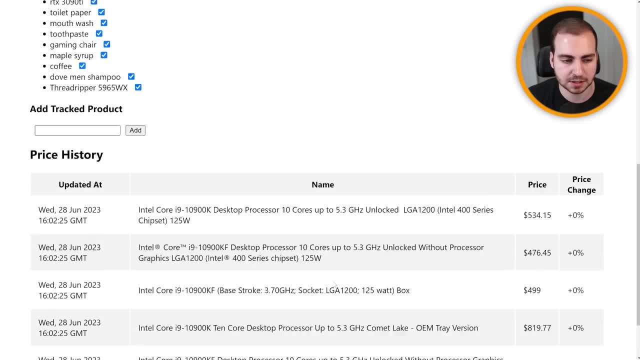 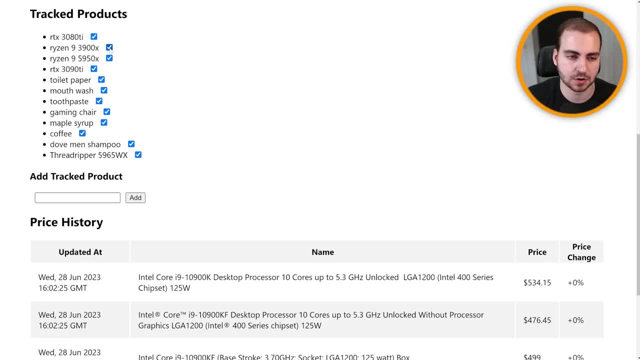 10, 900 K. So I can then run this every single day if I wanted to, And I could add this into my product list If I wanted to automatically run the scraper on it every few days. then again I can kind of go here and toggle them on or off If I know what longer want to track a specific. 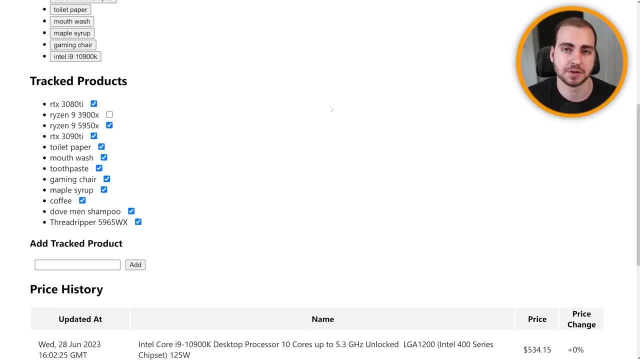 product. obviously a lot more stuff you can do here, but you see we have a very solid base setup. So now let me hop over to the code. I'll give you a bit of information on how this code functions, So you have some insight on how you could maybe change this if you wanted to work. 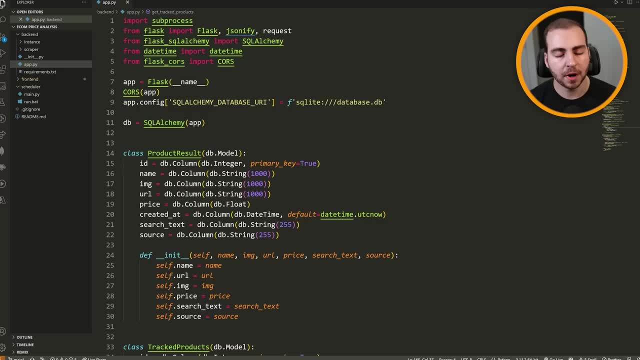 on a project similar to this. All right, So I've just hopped over to the code here and I'm just going to give you a very quick overview of the architecture of the product list. So let's go ahead and get started. So let's go ahead and get started. So let's go ahead and get started. So let's go ahead. 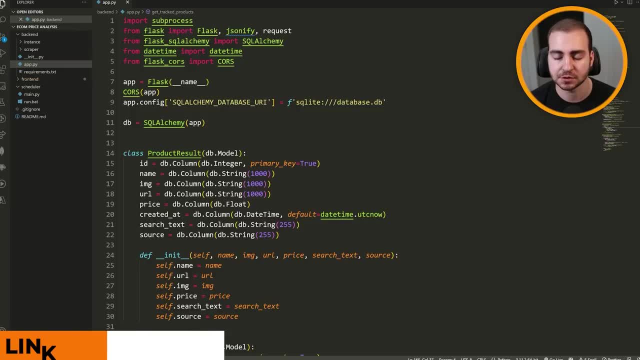 of this project And then again feel free to look at the code from the link in the description and extend this as you see fit. What I have for this is kind of three or four main components. I have a front end that's written to react. I have a backend that's written in flask with Python. 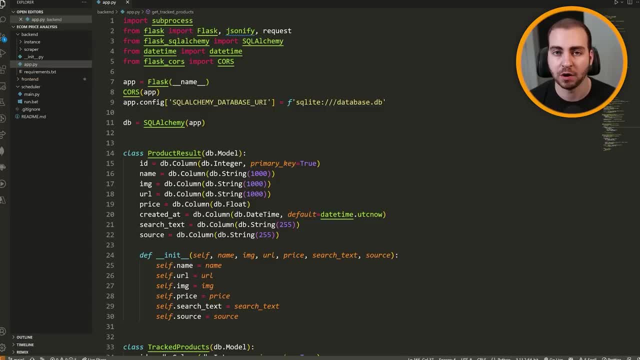 And then I have the actual scraper, which is a separate process. I run from my backend That's written in Python and uses playwright. I also have an automation script which is very simple and just automatically sends a API request to my backend every day. Now you 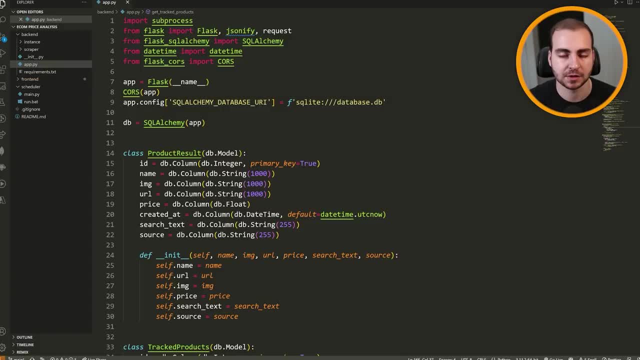 can set this every hour, every minute. You can use a cron job, You can use all kinds of stuff. but that's kind of how I've set this up. So I'm just going to walk you through very briefly the backend and then the web scraper, and we'll kind of go from there. Okay, So in my backend I have my app. 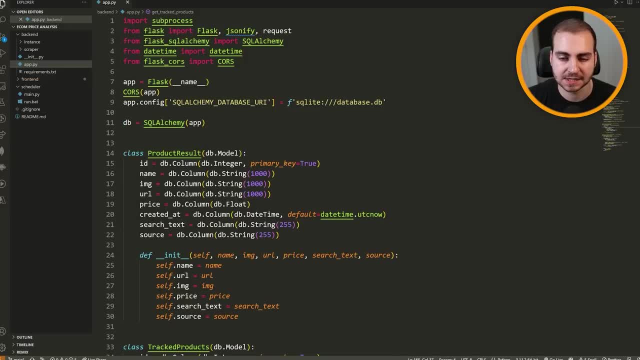 dot PI haven't organized this a ton And what I do is I set up here or I connect to a local SQLite three database. This is what I'm using to store all of my data. Obviously, you could use something like Postgres or MongoDB, but this was the simplest for this project. I set up my different database. 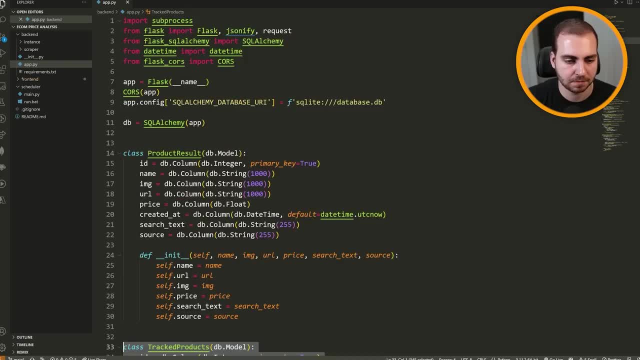 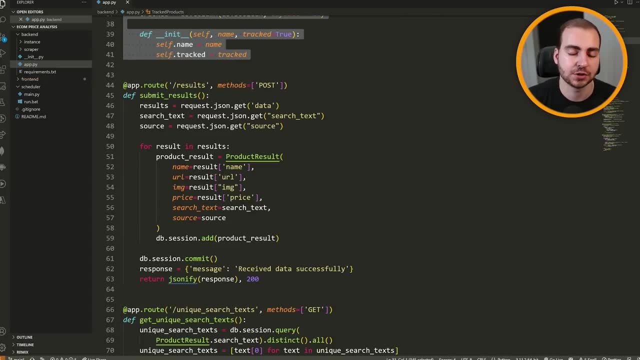 tables here, Yeah, Using kind of the SQL connector or SQL alchemy, whatever you want to call this in flask. And then I have a bunch of different end points. slash results is actually where the web scraper submits its results. So the API really allows the web scraper to interact kind of with my database and 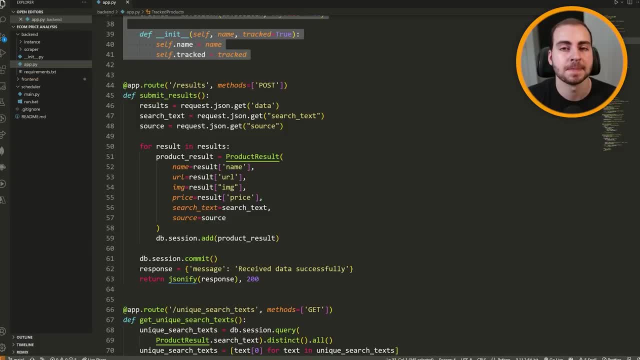 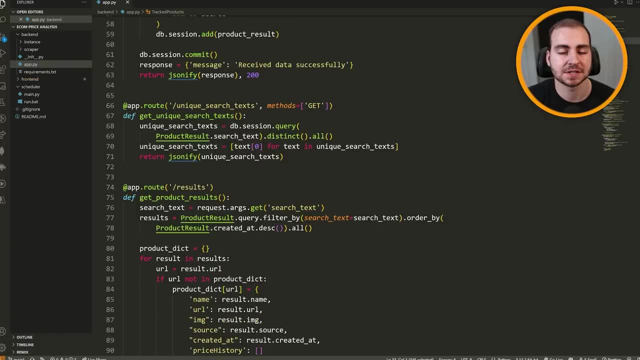 the backend. So I send a post request to results. that submits the results and then gets added to the database And then the front end can view that data. So that's what slash results is unique search texts. This is going to give all of the unique kind of searches that we've done. So the 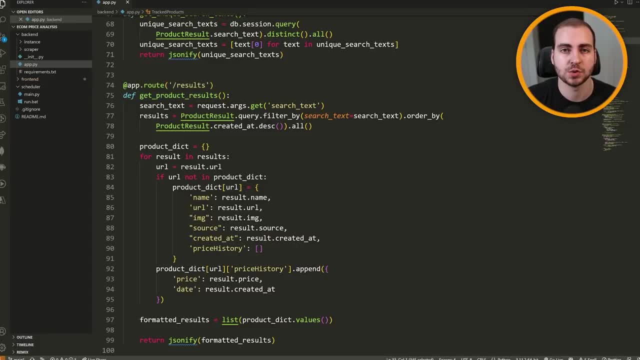 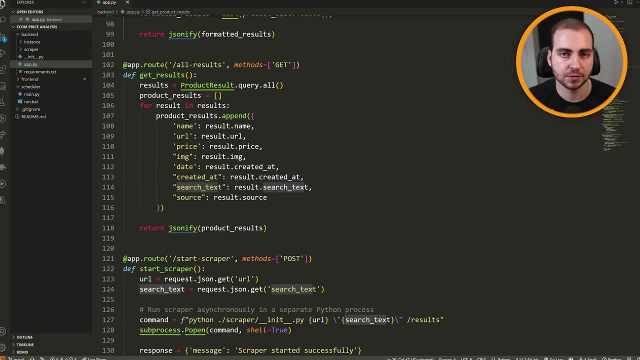 product names. essentially, we then have a get request here for slash results, which gives all of the results for a specific product name, which is the search text. We then have all results, which will give all of the results for all of the different products in our database We have start. 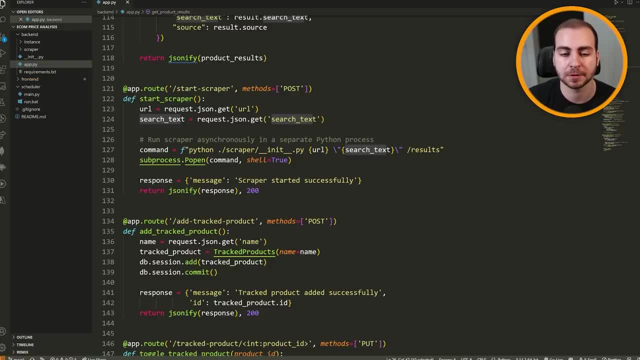 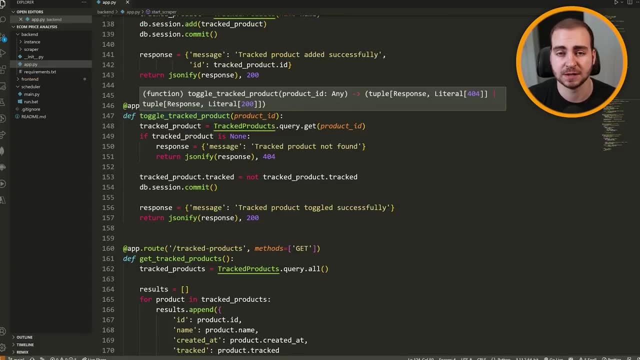 scraper, which is a post request method which is going to start the web scraper based on a URL and a specific search text. We have add tracked products straight forward. We then have a put for a tracked product which allows us to update it. So we can either toggle if we're tracking it or 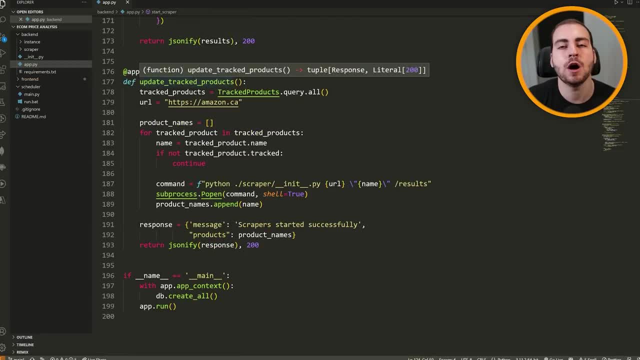 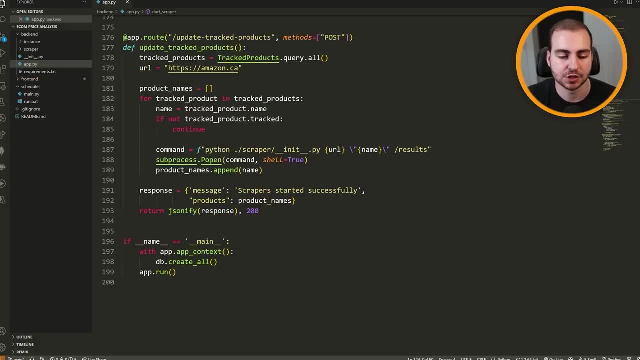 not. then we can have the ability to get all our tracked Products And then to update the track products, where what this will do is automatically run the web scraper on every single product instance. So you can see, what this does is create a new sub. 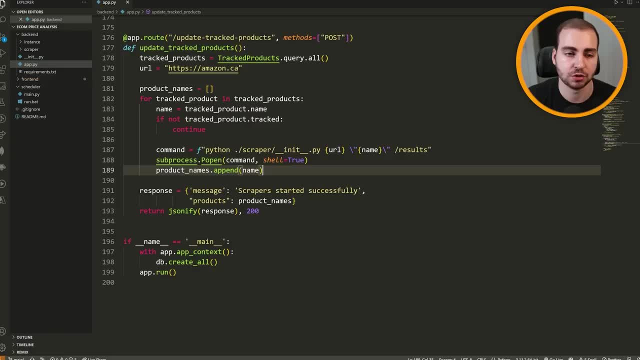 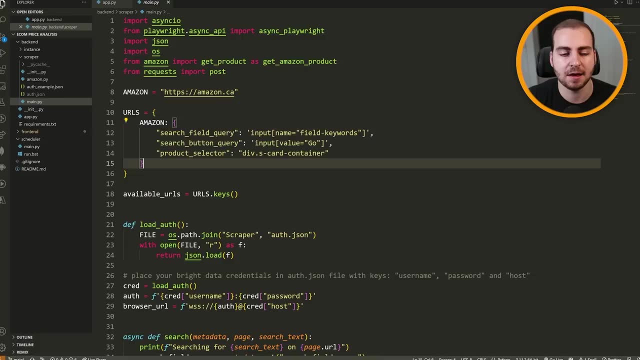 process where it then runs our Python scraper script, which I'll go into now. So I'm just going to very quickly kind of run through this. but I have this main dot PI file And what this does is kind of dynamically allow you to add different websites that you could be scraping. for now I've 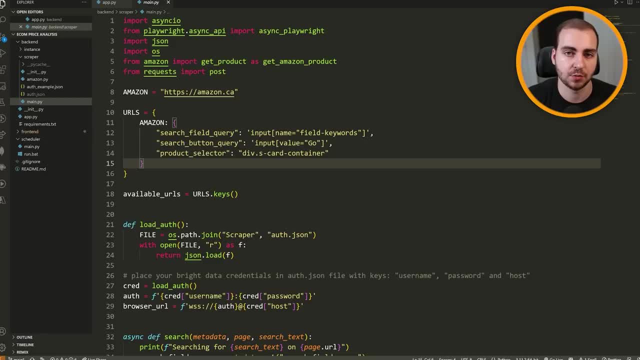 just set it up with amazonca, but you can connect this with really any website you want, So long as you write a very kind of specific piece of logic that will get the uh kind of elements that you're looking for, which I'll show you in one second. Now, what I do here is I connect right away to the bright data. 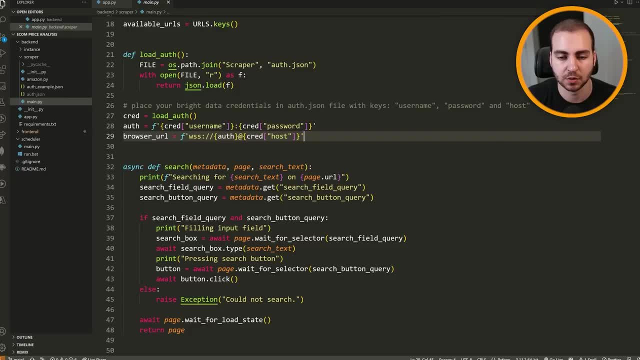 scraping browser. It's actually extremely simple. I was surprised how easy it was. All I do is just have to have my username, password and then my credential, which is what I get access to from my auth dot Jason file, which is inside of here, And then I just use that as the URL in play right. 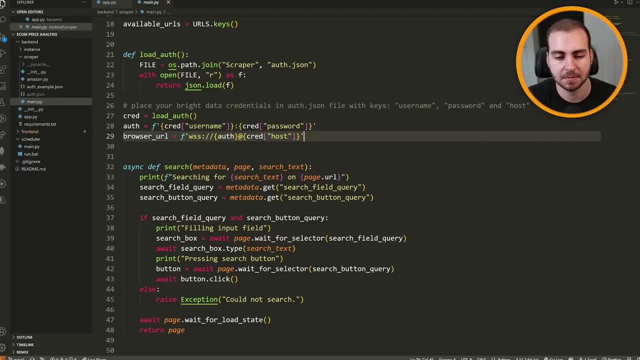 For the browser I want to connect to also works with puppeteer and Selenium, but it's literally like three or four Lines of code and you're automatically connected to the scalable network where you can run multiple instances of the scraper. So I won't really run through all of the text here, but you can see we 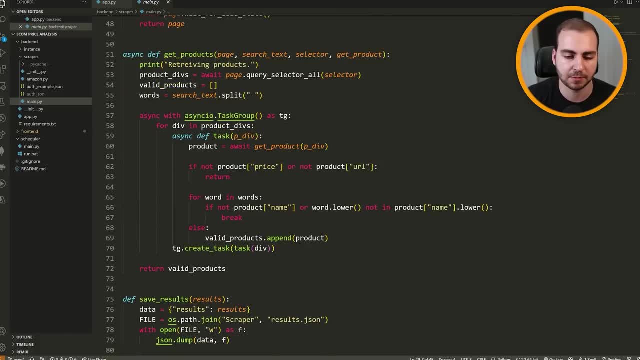 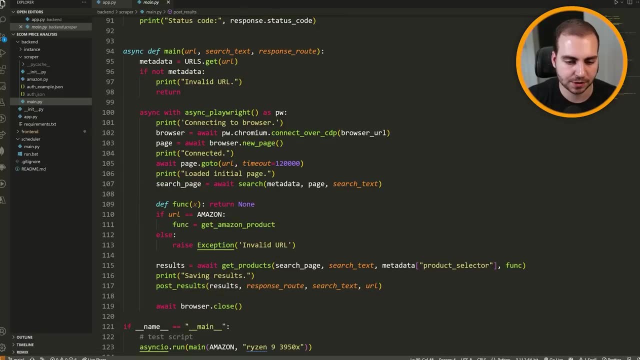 fill the input field, we press the search button, we retrieve the products, we grab all of that And then eventually what we do is we post the results here to our backend, where they get submitted to the database. Now, the core logic here is kind of connecting to the browser. So you can see, we're 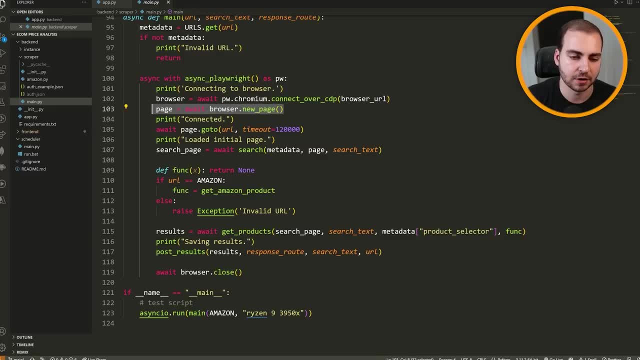 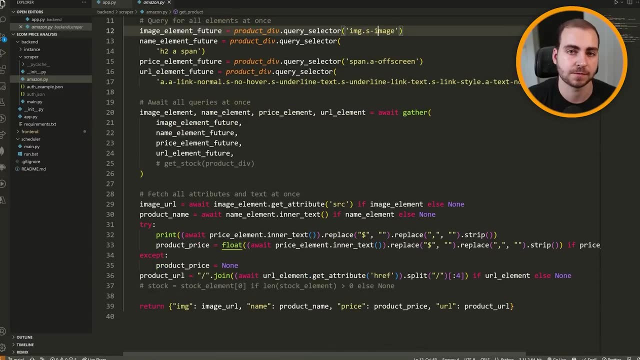 connecting over CDP to this browser URL: generate a new page, go to the URL You want to go to load the initial page, et cetera. We then have Amazon Pie, which is actually what's responsible for scraping the search page on amazonca. So it goes. 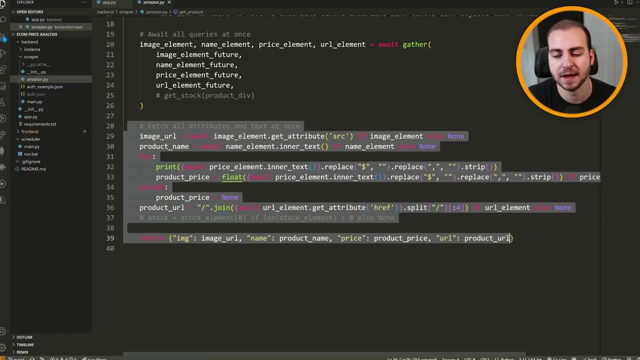 in gives us the image name, price, URL, get access to all of that and then just return that for each individual product. Obviously, there's a lot more logic that's going on here, but that's the basics and really everything that you need to know. So that's kind of how this works. Then I have my react. 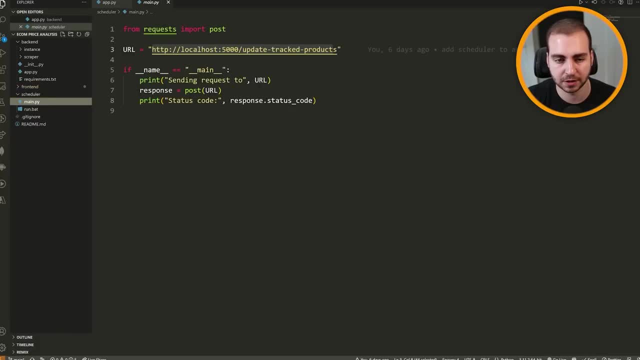 front end, Don't need to walk through that. And then, lastly, I have the scheduler here where all it does is just hit this URL here, So update track products once a day. the way this works that I've set up A windows batch file that I put in my windows process scheduler where every day it's automatically. 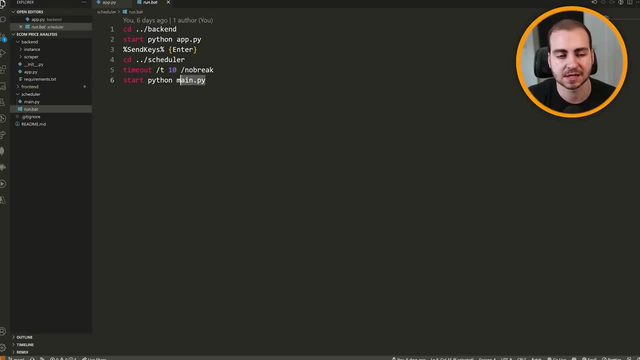 going to run this where it spins up the API and then it will wait 10 seconds and then call Python main up high- which is right here- which will send that post request which will then go retrieve all of the different products which will be spun up in parallel in separate processes. 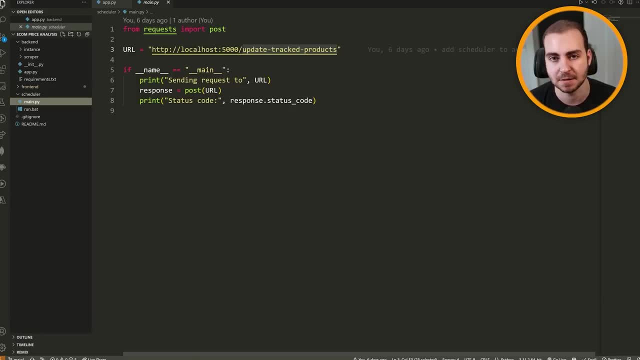 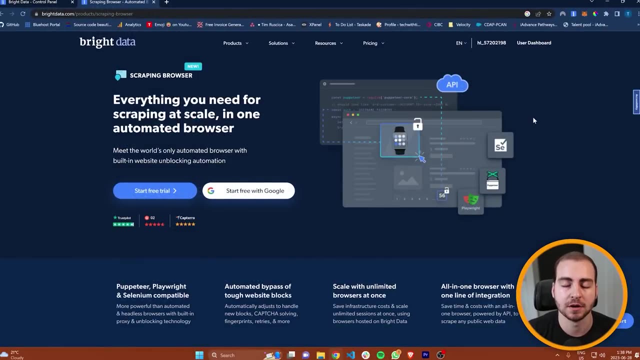 where we are scalably grabbing all of this data and adding it to the API. Now, just to quickly show you, in case you want to do this for yourself, what you would need to do is go to bright data, create a new account. 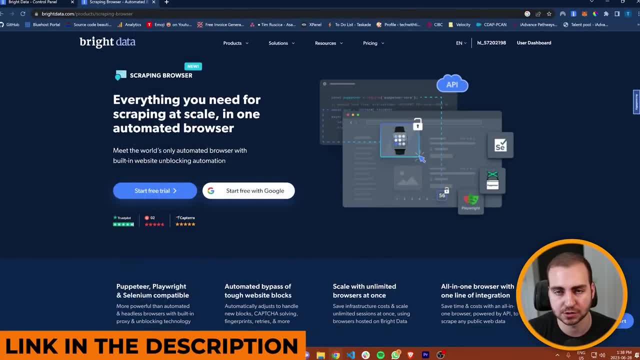 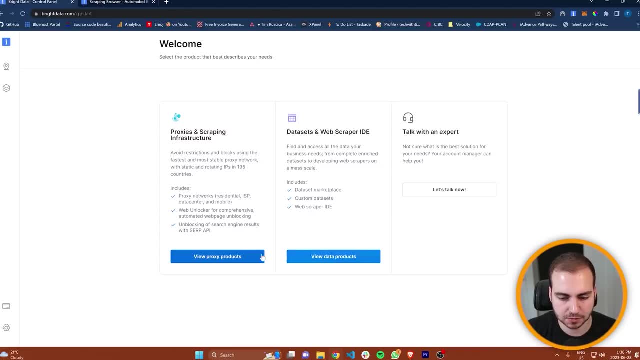 You can do that from there- The link in the description- and access the scraping browser. I'll leave some links in the description, but you can see it kind of gives you some information here. So from bright data go in, I'm going to go to my proxies and scraping infrastructure.